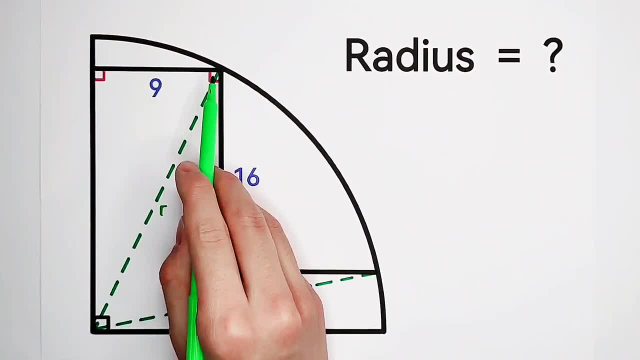 see, we've already got a right triangle over here. in this right triangle the hypotenuse is actually R and the short right angle side is 9. what about the long right angle side? we don't know. so now we have to solve for the length of. 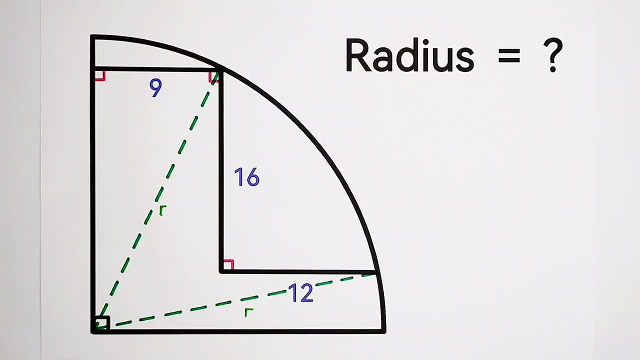 this side of the triangle. it's not easy. but now, if we extend this line segment to here, what can we get? so now we can find out that these two angles are right angles, then this is actually a rectangle. in any rectangle, the two opposite sides are always equal and parallel to each other. so that means here is 16, here as. 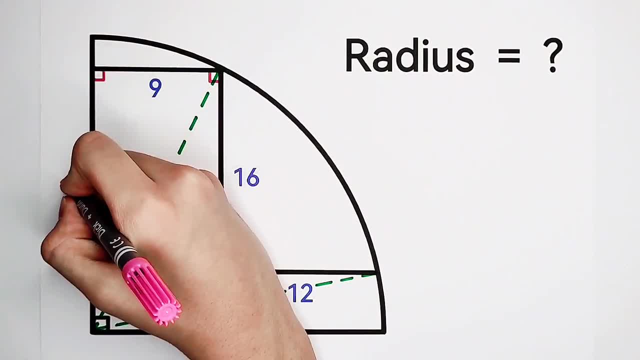 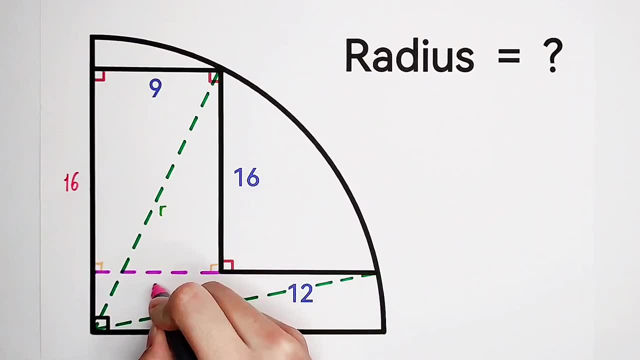 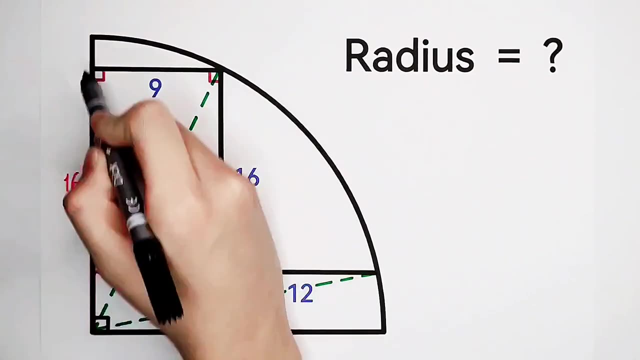 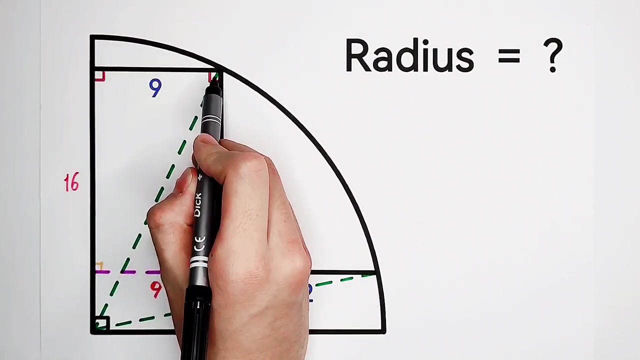 well, 16, and here is 9, here as well. now we've actually got two right triangles and these two right triangles are this one and this one in this right triangle. this side is known 9, it is given hypotenuse is R, we supposed, and the long right angle side is still very. 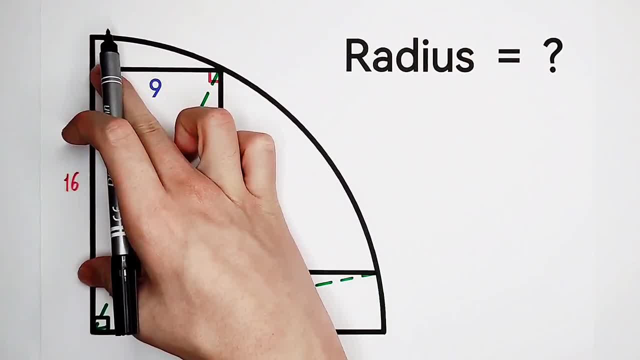 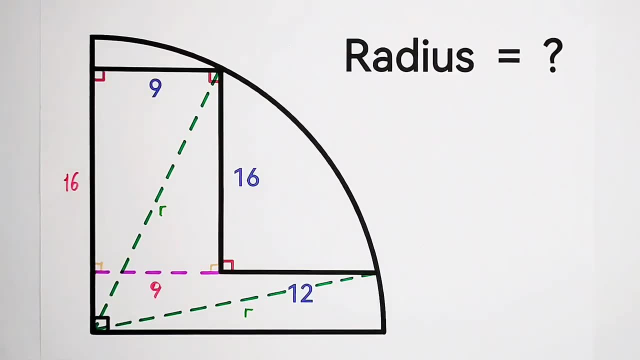 strange because we've only known that this section measures 16, so now we lack this part, this small section in our this right triangle. hypotenuse is R. long right angle side is 12 plus 9 is 21. however, the short right angle side is a mystery. here this small guy appears in. 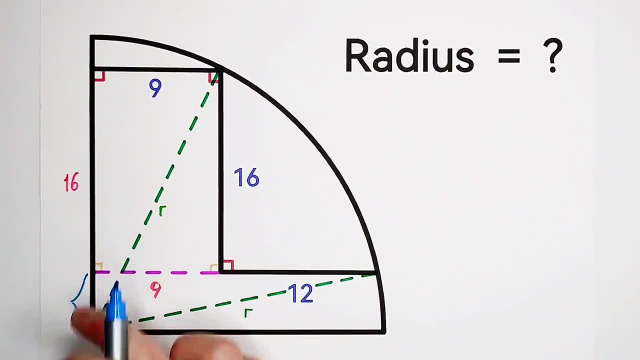 both right triangles and we have to know its length, which I'll do, of course. we can suppose again. we can suppose that this small section measures, for example, X, then, because we have two right triangles, so in these two right triangles we can use the Pythagorean theorem two times. in this one it is. 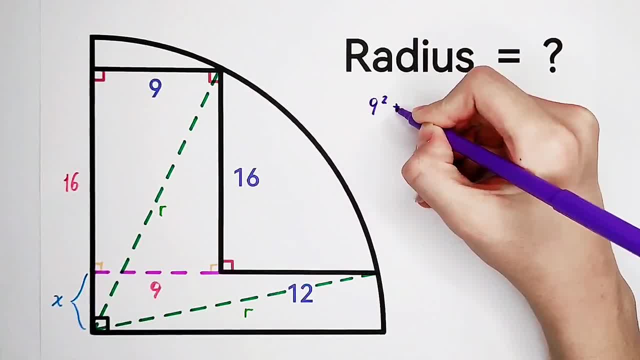 two right triangles, so we can use the Pythagorean theorem two times in this one. it is two right triangles, so we can use the Pythagorean theorem two times in this one. it is basically two great triangles and we can use the Pythagorean theorem two times in this one it is. 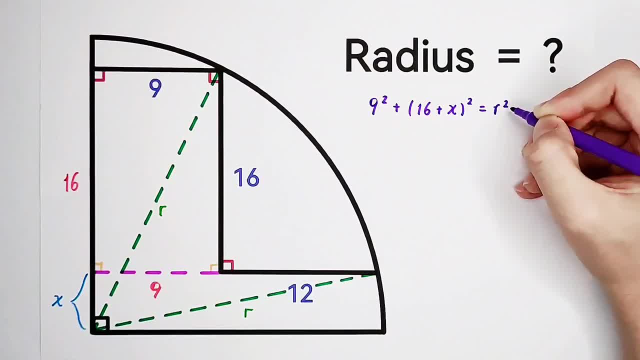 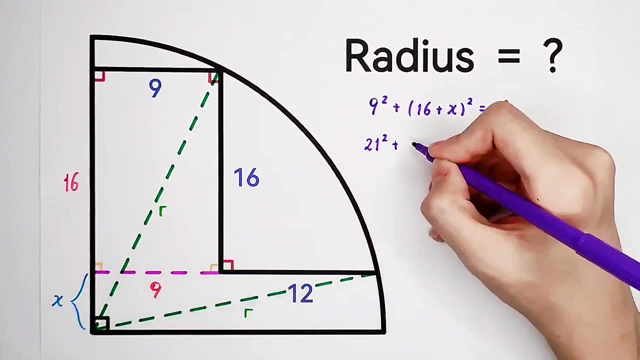 also this part, and it is actually quite expensive, and in a regular percentage way, we would still use these pieces. it should be very cost effective. here is theicked value of a girl who is 18 Waldenín steps. It's I. So now, how can we solve this system of equations? 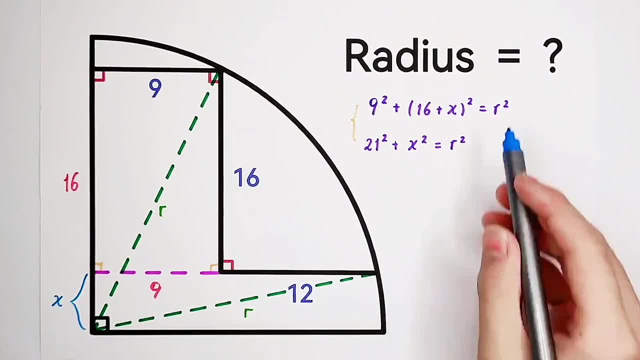 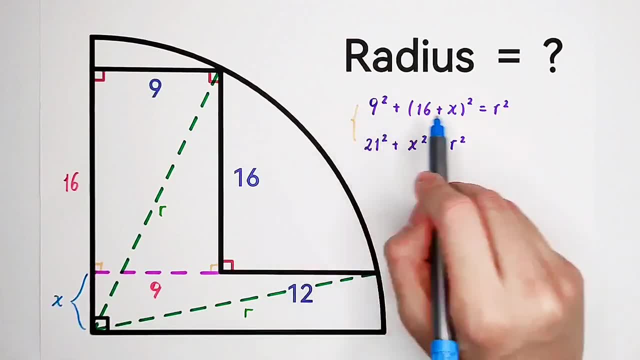 I hope that you can immediately find out that the right-hand sides are the same: r squared, r squared. So now, what does it mean? This guy equals r squared. this guy is also equal to r squared. Of course, that means the two left-hand sides equal each other. 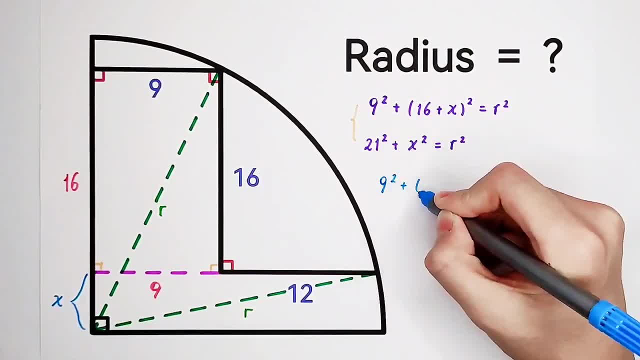 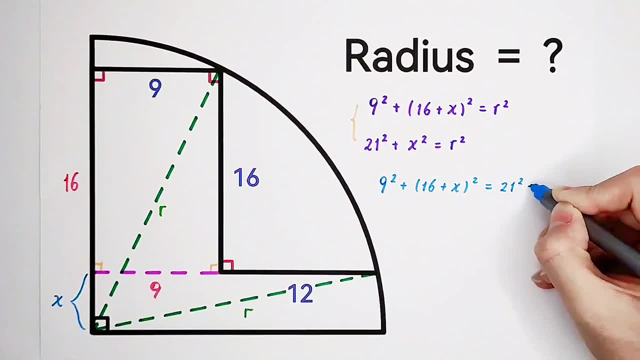 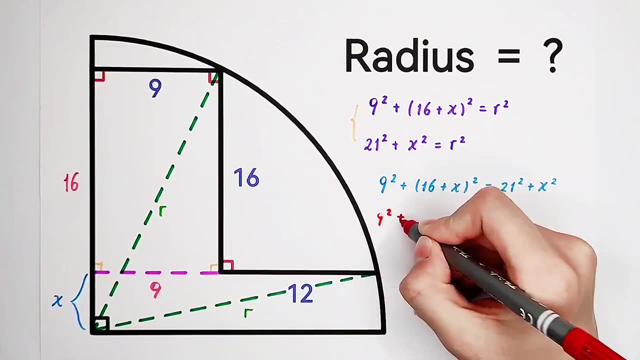 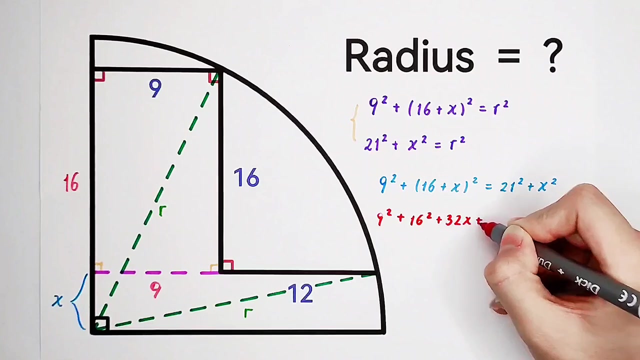 So it's just 9 squared plus 16 plus x. all squared equals 21 squared plus x squared. Now the only thing we can do is to expand this guy: 16 squared plus 32x. Okay, 21 squared plus x squared. 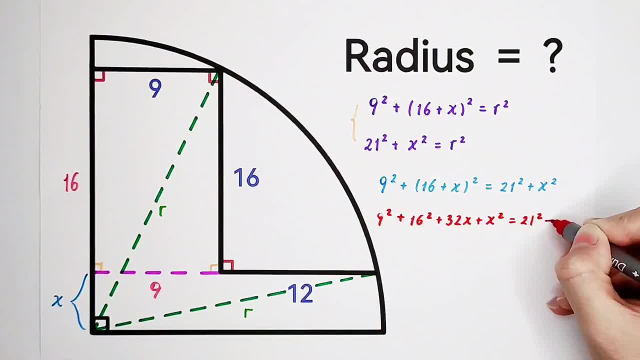 And the right-hand side is still 21 squared plus x squared Now. congratulations: Plus x squared, plus x squared- cancel. Now 32x is actually 21 squared minus 9 squared, minus 16 squared. I don't know if there exists a trick. 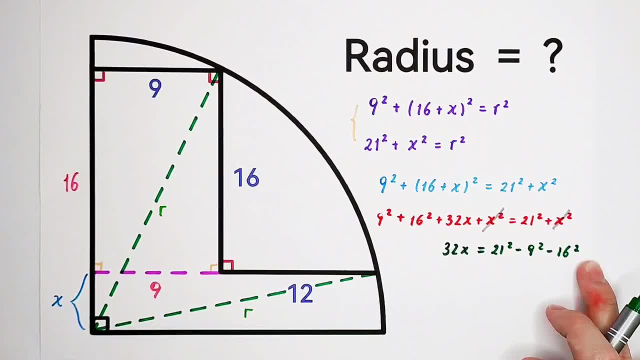 If not, Just calculate the right-hand side and divide it by 32. Then you can evaluate x. The value of x is just 13 over 4.. Oh, rational, isn't it? We have to solve for the length of the radius. 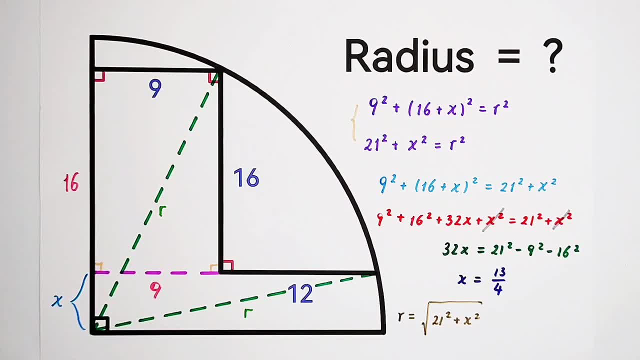 Because r is the radius and radius is the length, and every length is non-negative. So of course r has to be the positive root, So r has to be the negative root of 21 squared plus x squared. Then we can find out that the answer is very, very rational.